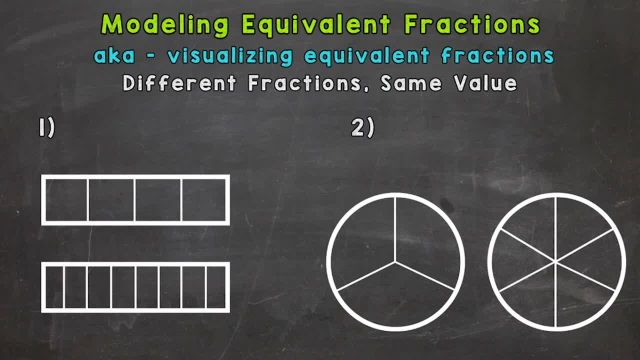 number one, where we have two rectangles that are the exact same size but they're cut into a different amount of pieces. So the top rectangle is cut into fourths and the fraction we're going to start with is three-fourths. So let's model three-fourths. This would be one-fourth. 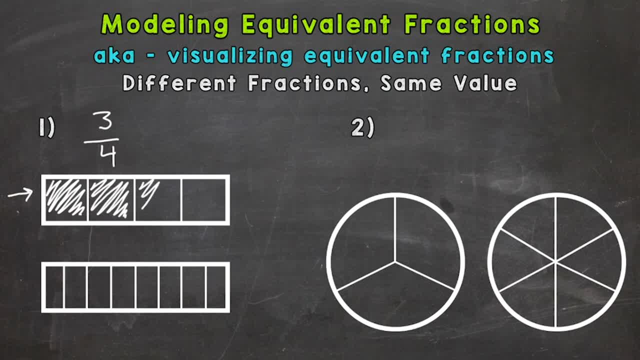 two-fourths and finally three-fourths, So that top rectangle represents three-fourths. Now we need to create an equivalent fraction with that bottom rectangle, which is cut into eighths, So we need to fill it in the same exact amount. So, for example, if we filled it in one-eighth would. 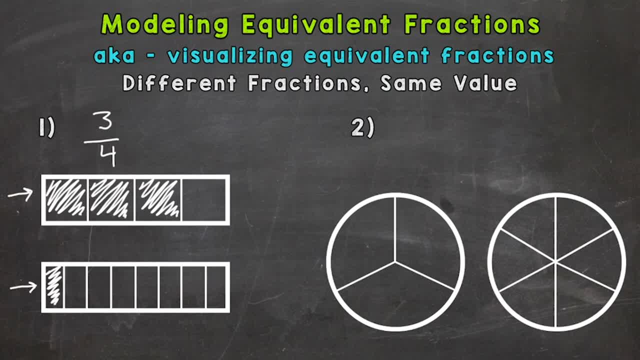 we be filled in the same exact amount as the top rectangle. No, So let's keep going. Two-eighths, three-eighths, four-eighths, getting closer, five-eighths and six-eighths, And we can see. 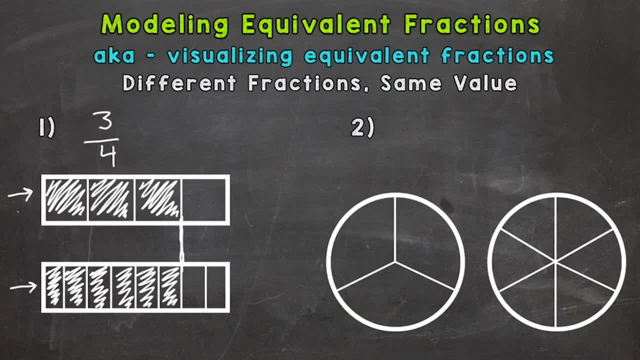 that they're filled in the same exact amount here. So the equivalent fraction is six-eighths. Now we modeled those equivalent fractions. Now, in order to find equivalent fractions, you don't have to draw a model every time. I dropped a link to the video where I 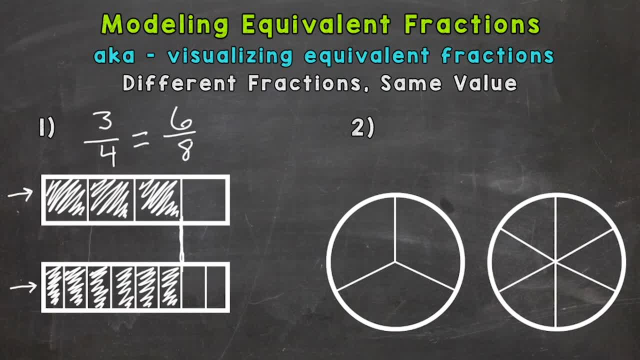 explain how to find equivalent fractions without models down in the description. But again, this video is about visualizing and seeing what equivalent fractions look like. So let's take a look at number two, where we have two circles that are the same exact size but cut into a. 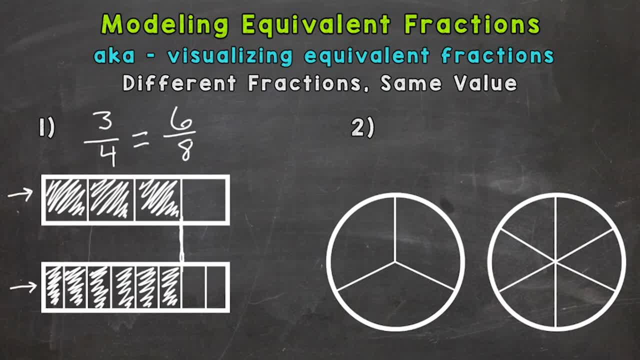 different amount of pieces. So let's look at number two. We have twoiovual. Now we have two of the. so the first circle on the left is cut into three pieces or thirds. so let's fill in one of those pieces and that will represent 1- 3rd. so we just modeled. 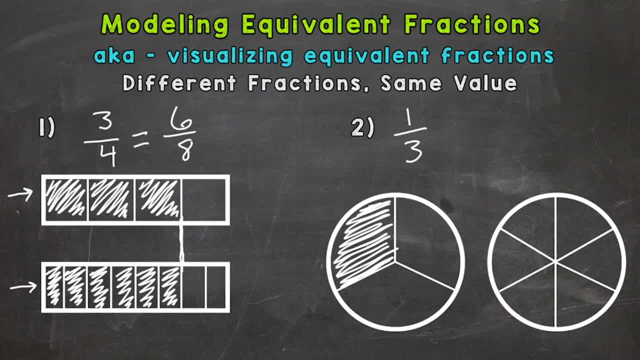 1. 3rd, and the circle on the right is cut into six pieces, so sixths. let's fill in one out of six to see if we get an equivalent amount of space filled in and therefore an equivalent fraction. not quite, so let's fill in two sixths or two.